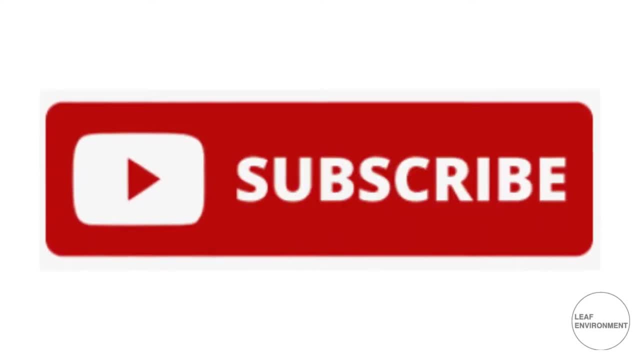 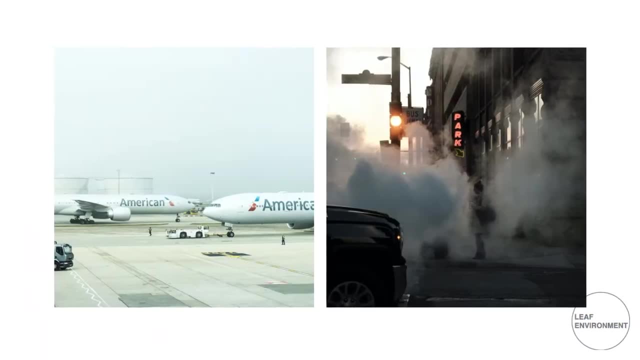 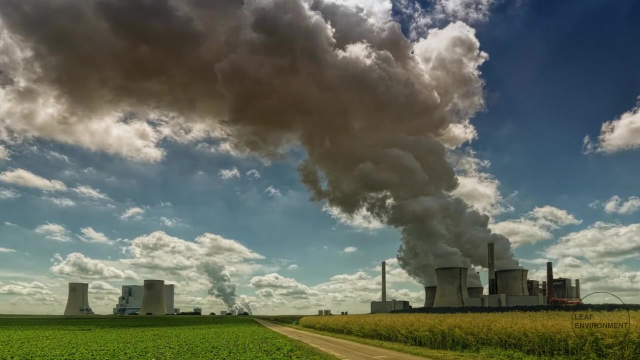 Please subscribe to my youtube channel. leaf environment into today's world. air pollution is one of the biggest threats for the environment and affects everyone: humans, animals, crops, cities, forests, aquatic ecosystems. what causes air pollution, what are the effects and, most importantly, what are the possible solutions to tackle it? air pollution can be defined as: 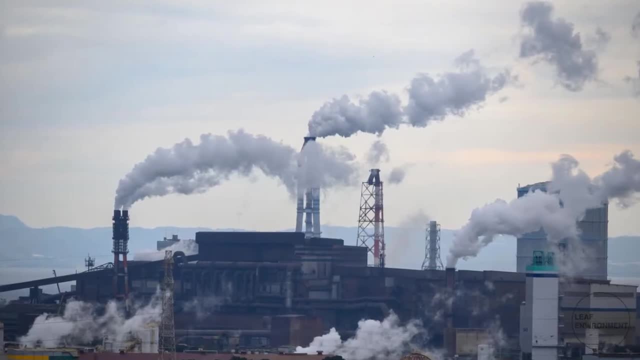 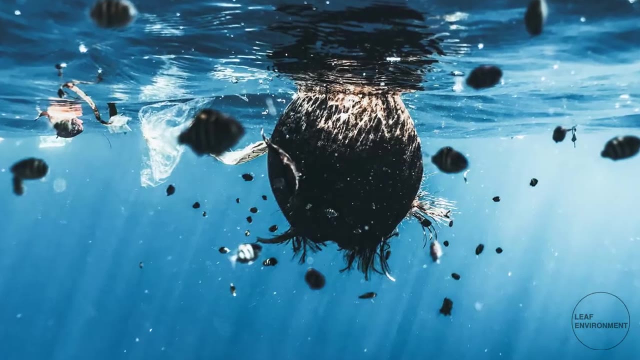 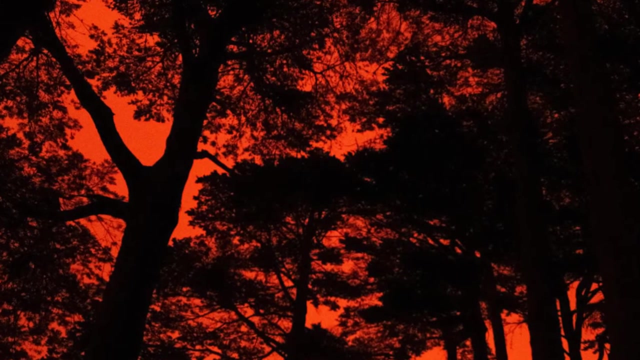 an alteration of air quality that can be characterized by measurements of chemical, biological or physical pollutants in the air. therefore, air pollution means the undesirable presence of impurities or the abnormal rise in the proportion of some constituents of the atmosphere. it can be classified in two sections: visible and invisible air pollution. 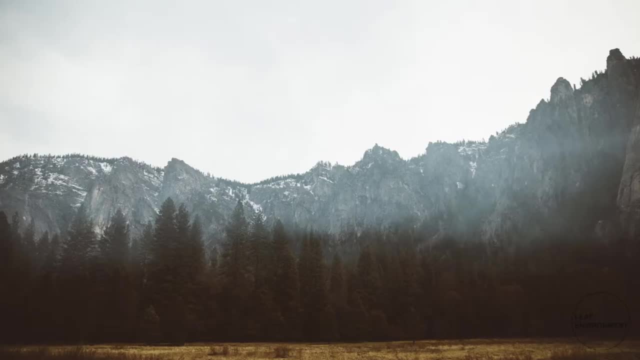 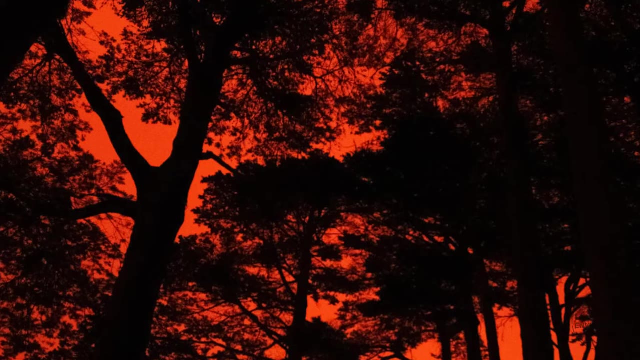 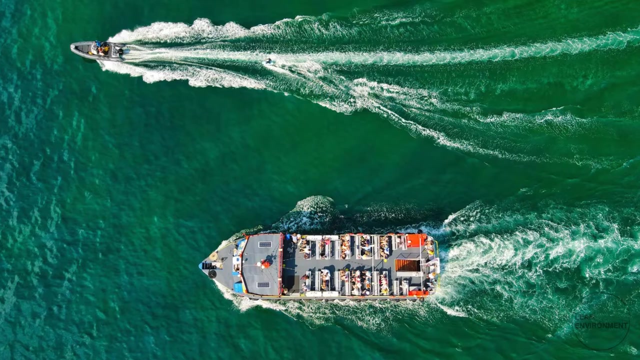 air pollution is caused by the presence in the atmosphere of toxic substances mainly produced by human activities, even though sometimes it can result from natural phenomena such as volcanic eruptions, dust, storms and wildfires, also depleting the air quality. air pollution sources are: first, combustion of fossil fuels like coal and oil for electricity. 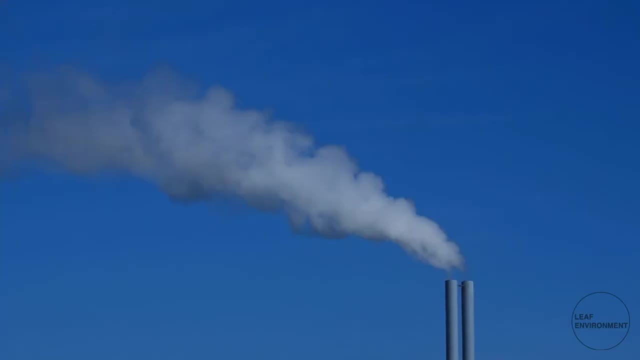 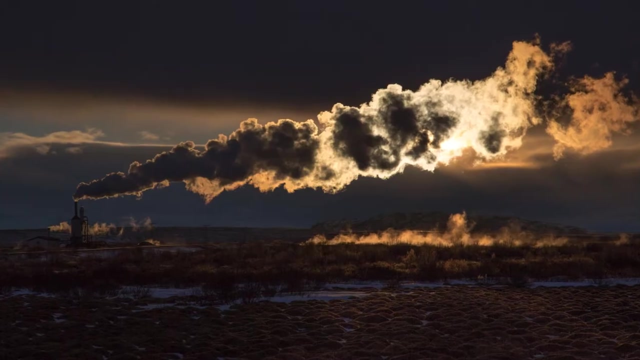 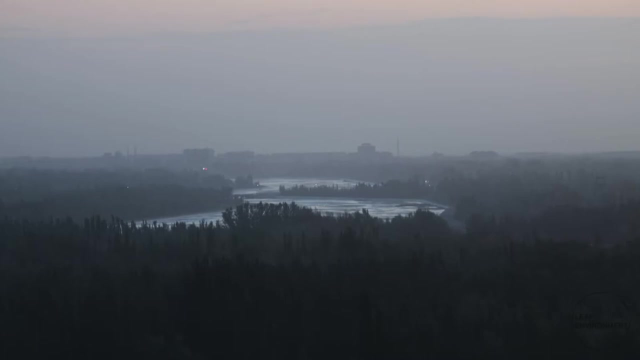 and road transport, producing air pollutants like nitrogen and sulfur dioxide. second, emissions from industries and factories, releasing large amount of carbon monoxide, hydrocarbon, chemicals and organic compounds into the air. third, agricultural activities due to the use of pesticides, insecticides and fertilizers that emit harmful chemicals. 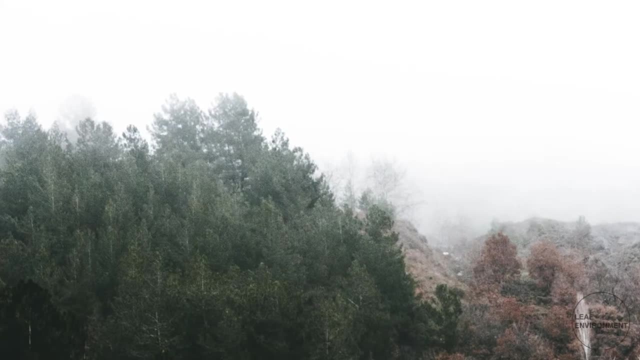 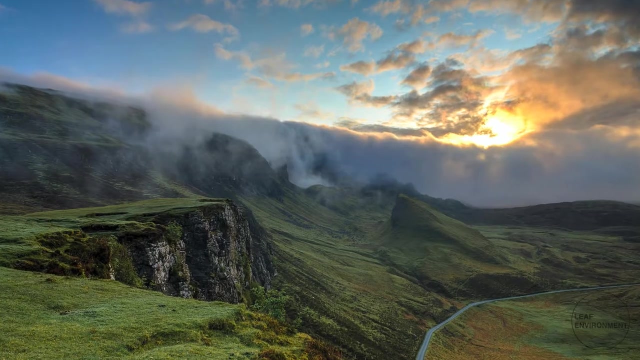 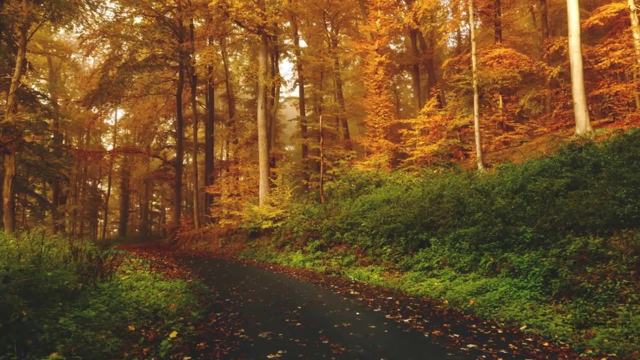 fourth, waste production, mostly because of methane generation in landfills. it is impossible to describe the whole extent of potential and actual damage caused by all forms of air pollution, but here are the main consequences. air pollution has a major impact on the process of plant evolution by preventing photosynthesis, in many cases with serious consequences for the purification of the. 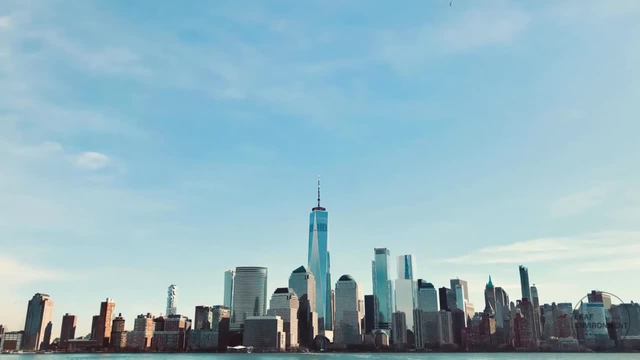 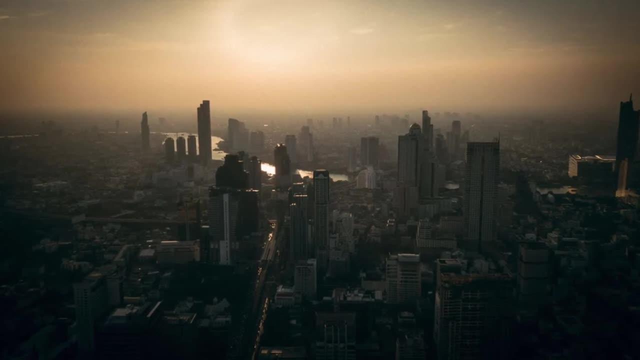 air we breathe. it also contributes to the formation of acid rain. atmospheric precipitations in the form of rain and the formation of acid rain is also a major consequence of the formation of acid rain. the space moving between water humps and the soles of the land on top now in some locations to 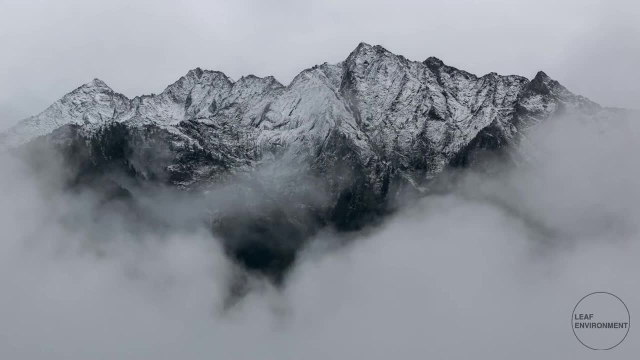 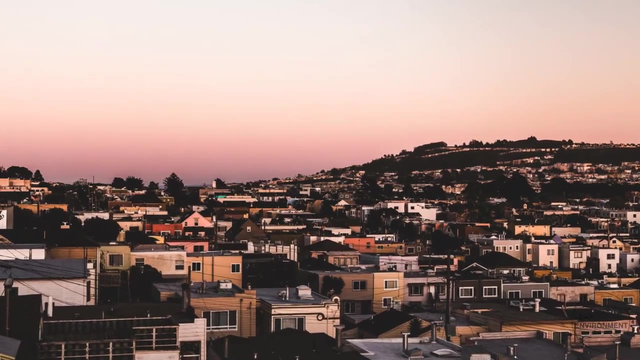 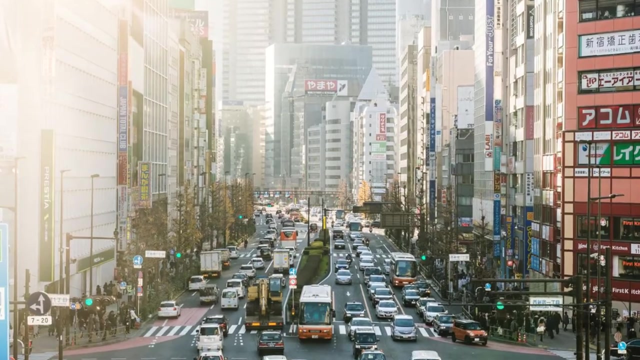 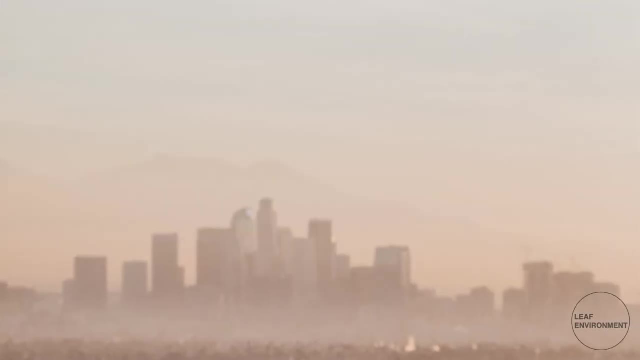 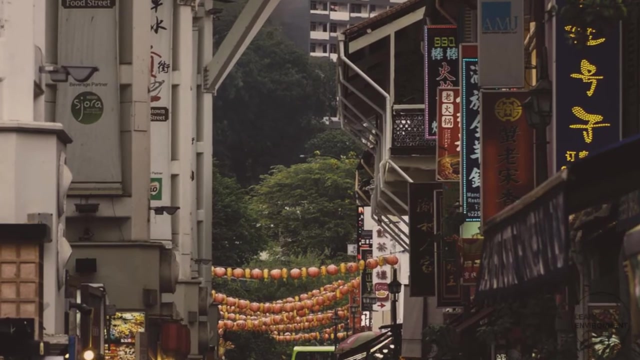 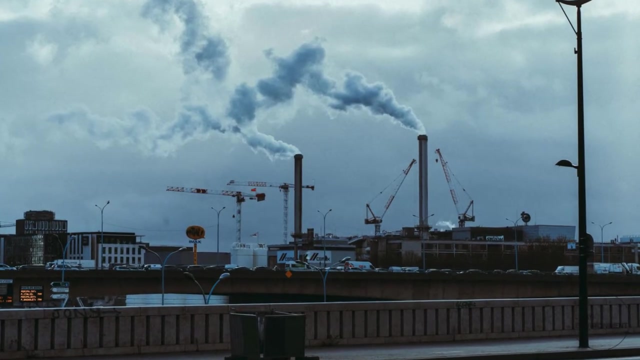 the cause of the recent climate change on human health. our continual exposure to air pollutants is responsible for the deterioration of human health. air pollution is indeed a significant risk factor for human health conditions, causing allergies, respiratory and cardiovascular diseases, as well as lung damage. air pollution prevention: there are ways to prevent, control and, eventually, 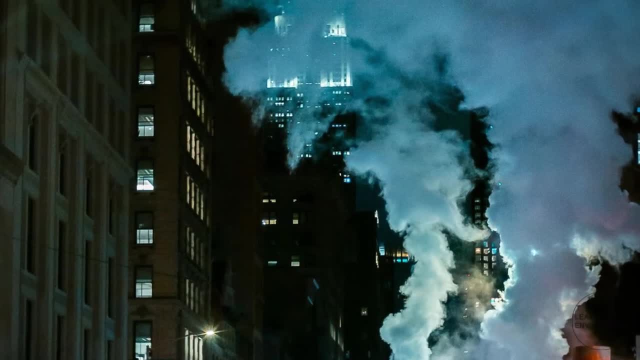 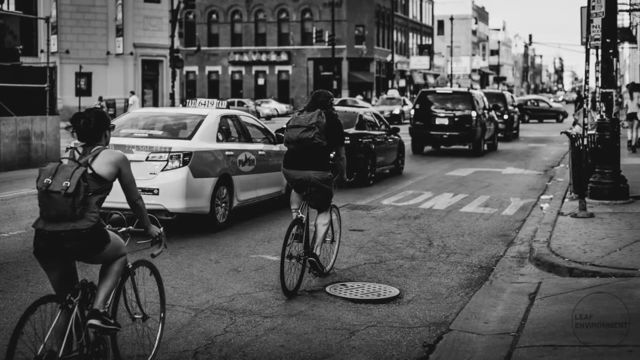 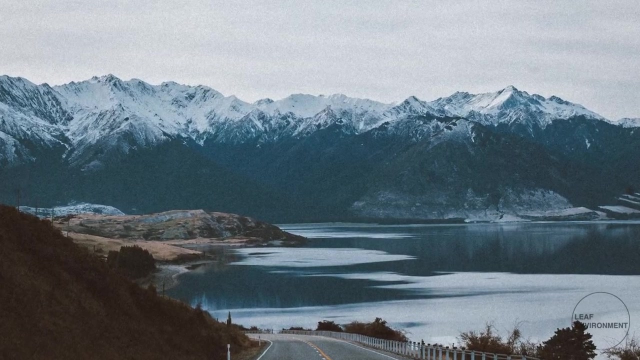 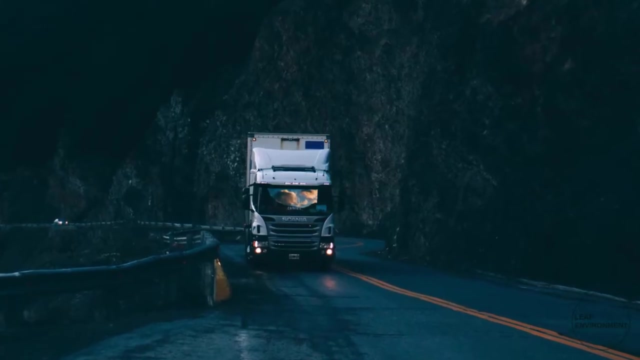 reduce air pollution, one renewable fuel and clean energy production. the most basic solution for air pollution is to move away from fossil fuels, replacing them with alternative energies like solar, wind and geothermal two: energy conservation and efficiency. producing clean energy is crucial, but equally important is to reduce our consumption of energy by adopting responsible habits and using 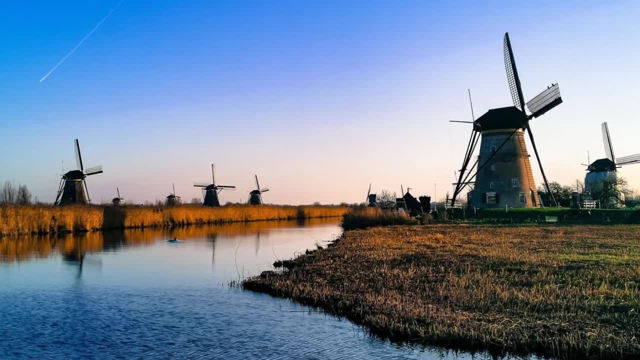 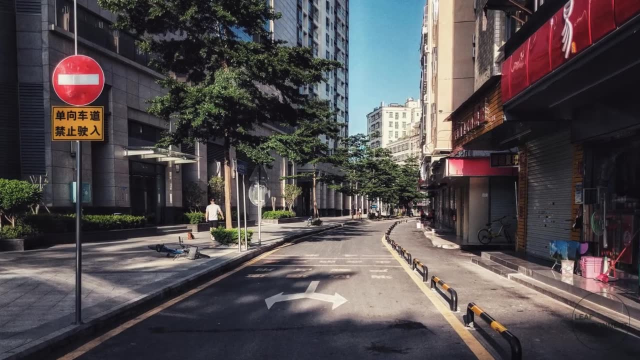 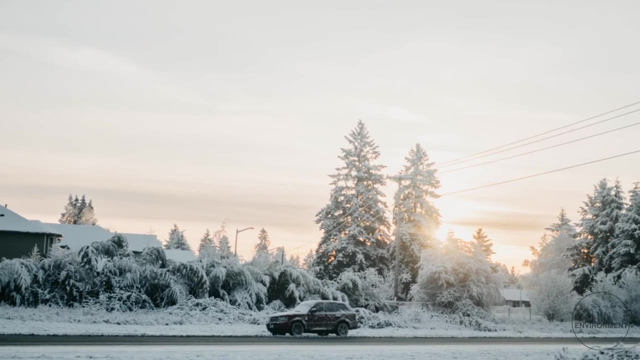 more efficient devices. three: eco-friendly transportation: shifting to electric vehicles and hydrogen vehicles and promoting shared mobility, ie carpooling and public transport, to reduce air pollution. four: green building: from planning to demolition. green building aims to create environmentally responsible and resource efficient structures to reduce their carbon. 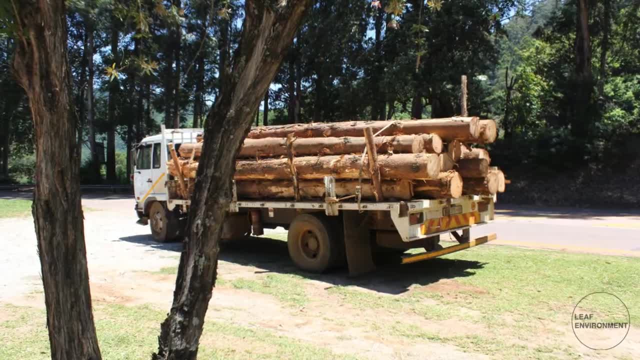 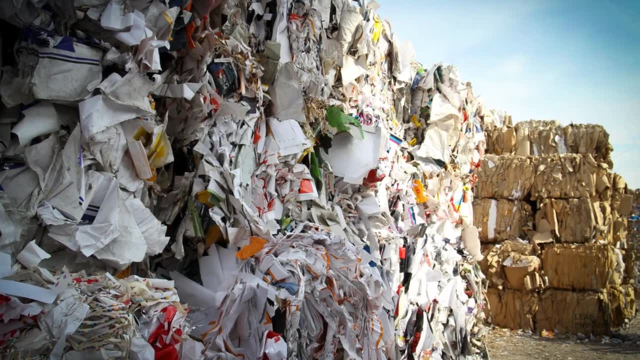 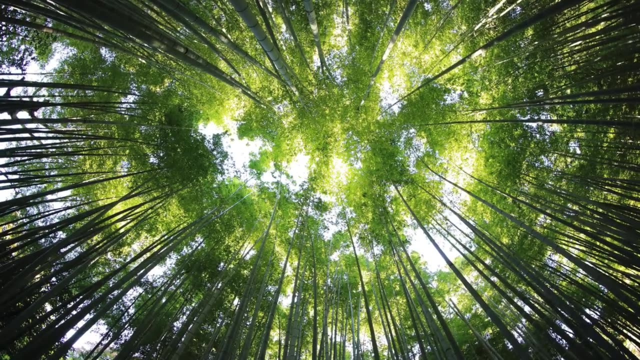 footprint. in addition, monitoring air pollution levels has become very important to detect pollution peaks, better control air pollution and eventually improve air quality. how is air quality measured? with measuring devices using laser-based technologies, chamois, luminescence, flame, ionization, etc. these devices are, for instance, located close to the traffic, far from the traffic and close to 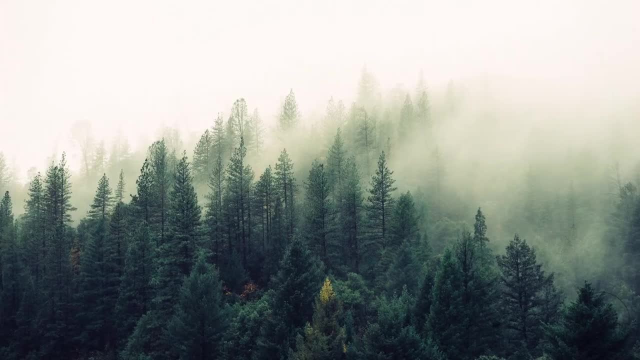 industrial zones. all the collected data are compiled into a value scale called the air quality index aqi. if you like my channel, then please subscribe and press like.